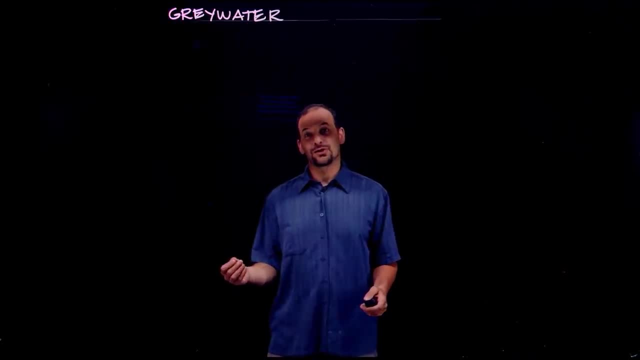 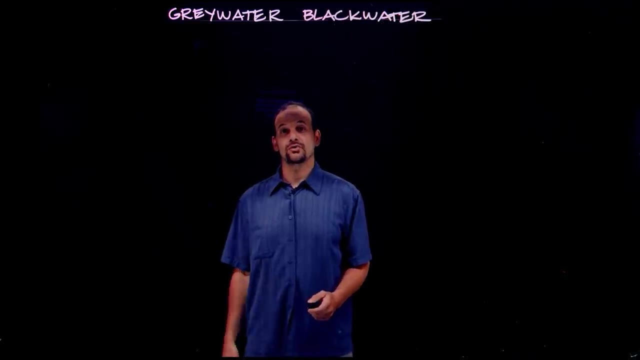 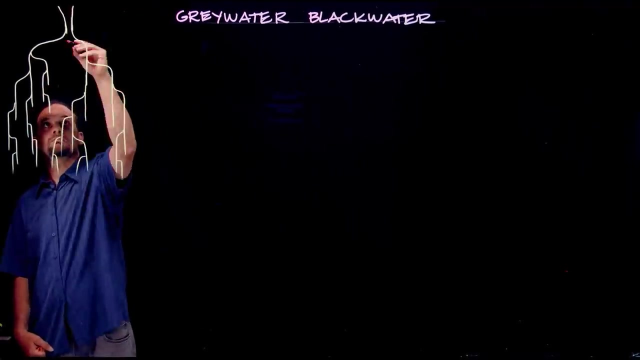 We're talking about gray water, which is the slightly dirty water from showers, laundry and sinks, And we're talking about black water, which is water from toilets and other really dirty uses. So let's start by looking at wetland plants, So the root systems of wetland plants. are like the roots of plants. So the root systems of plants are like the roots of plants. So the root systems of wetland plants are like the roots of plants. So the root systems of plants are like the roots of plants. So the root systems of plants are like giant festivals of microorganisms. 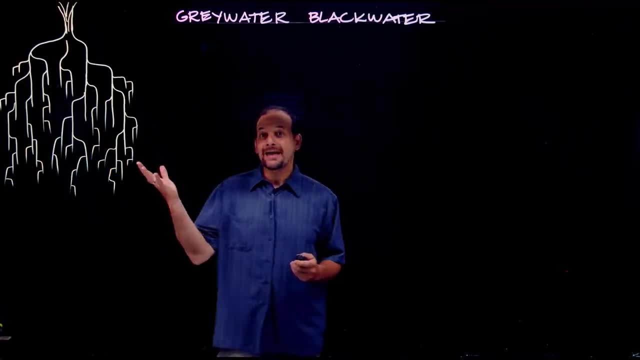 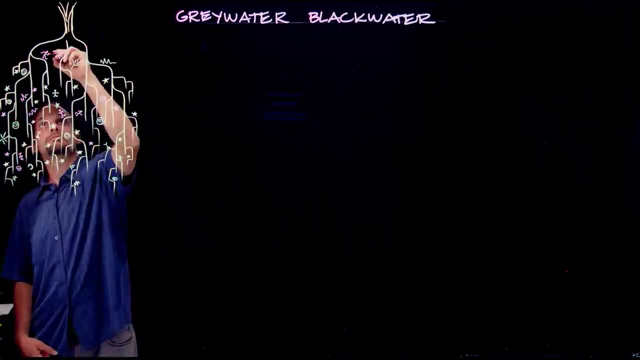 like bacteria and fungi, This massive microorganism party can actually biodegrade most minor pollutants, breaking them down into harmless elements. The microorganisms are partying on the roots, and the roots form this mat that becomes a living filter trapping sediment and 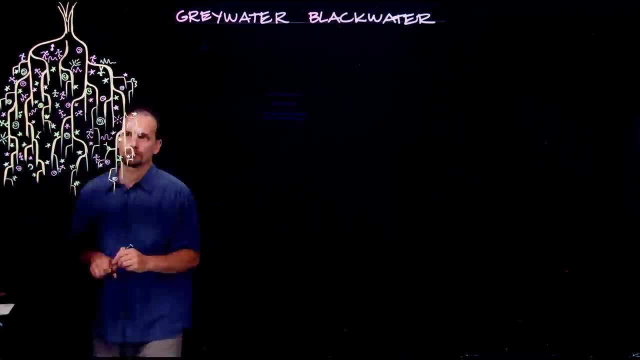 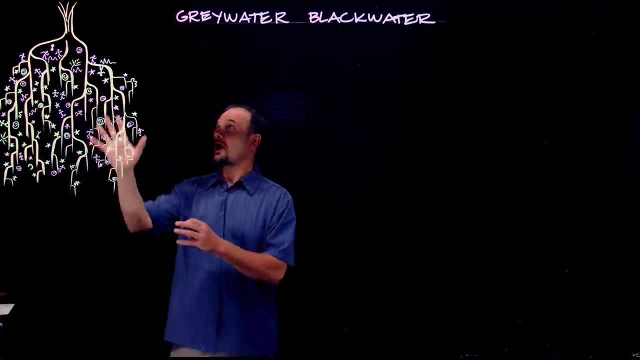 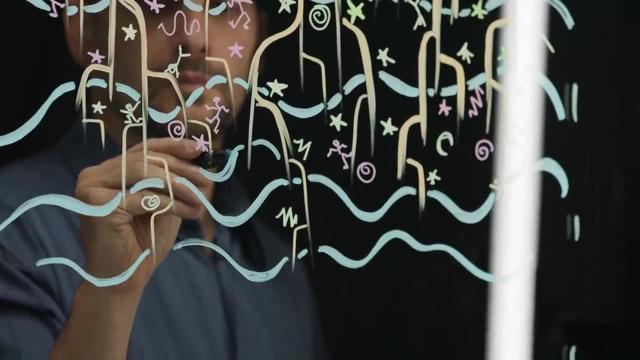 supplying food and drink for the festival of life. So in addition to this root filter, some wetland plants can actually absorb heavy metals from the water up into their tissues. So the goal of any wetland water treatment system is to create the maximum amount of contact between 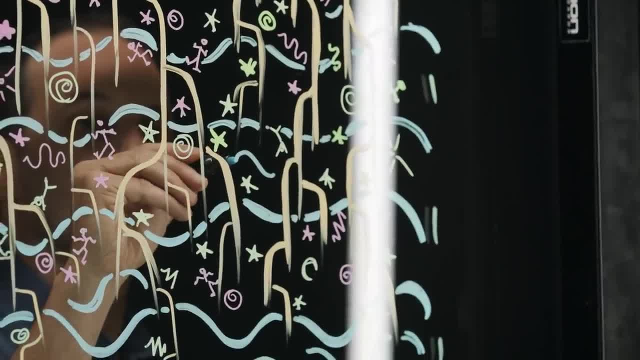 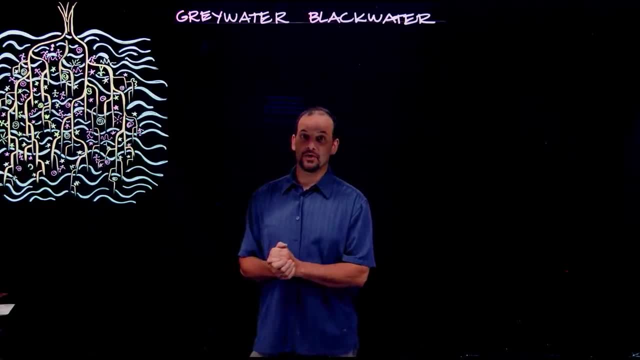 the dirty water and the roots of a diversity of plant species. So the very simplest version of how this concept is used in wastewater treatment is the constructed wetlands. So in this example, wastewater flows through the soil. So in this example, wastewater flows through the soil. So 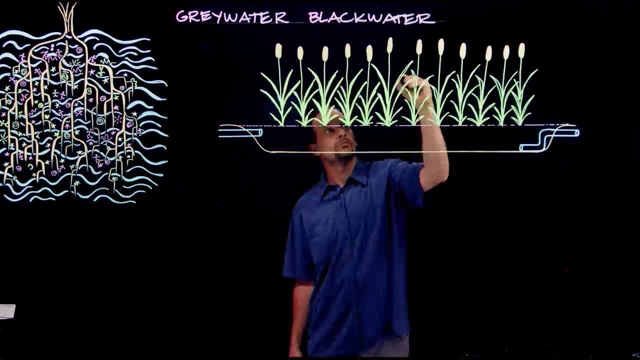 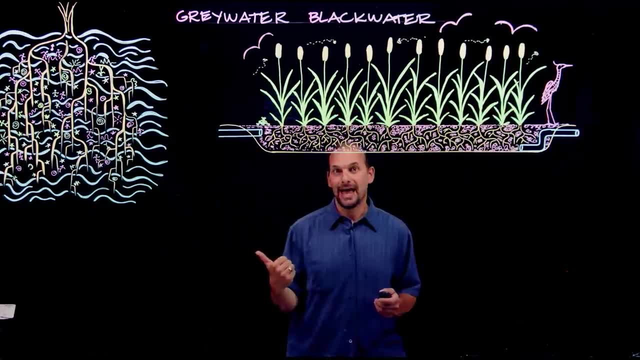 in this example, the wastewater flows into this gravel-filled basin that's planted with wetland plant species and is lined on the bottom with either plastic or cement or some other material. so the water doesn't seep into the ground but stays in this container here. So the water flows. 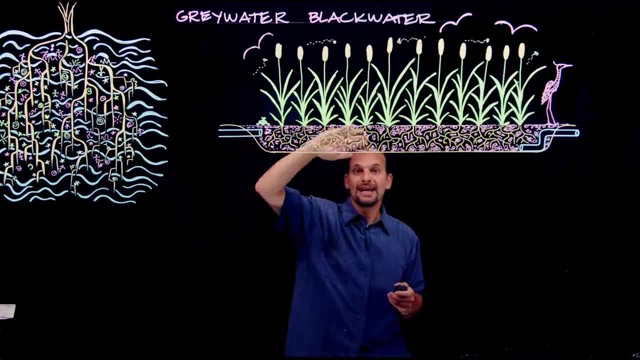 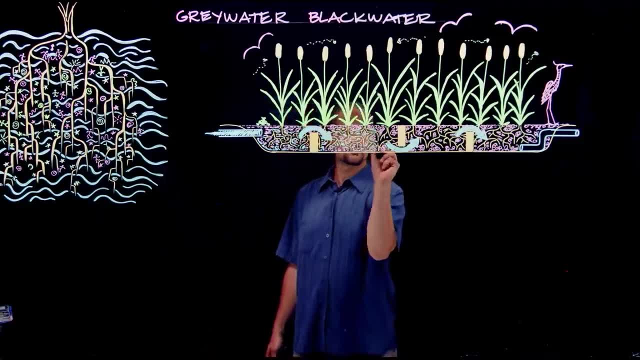 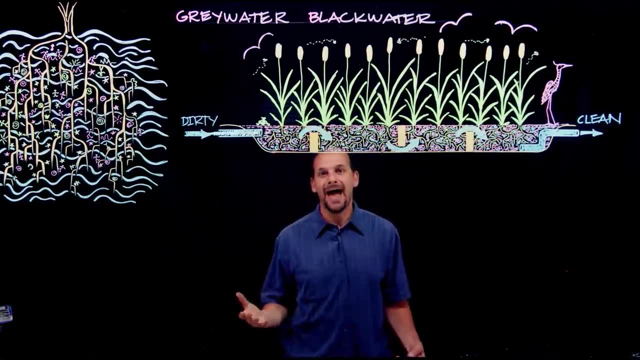 underneath the gravel level, so dirty water is never exposed to the air. Now you can also place some sort of baffles in the system. So you can also place some sort of baffles in the system so that the water is forced to move up and down through the system, ensuring maximum contact with 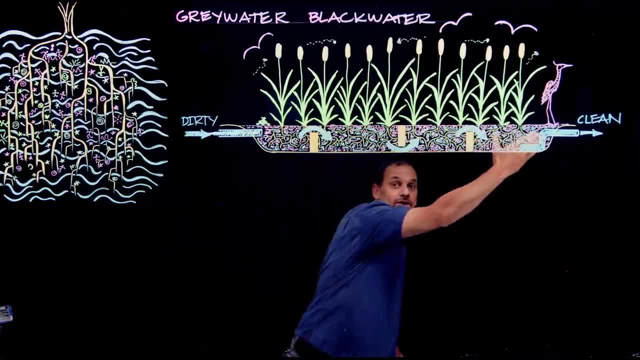 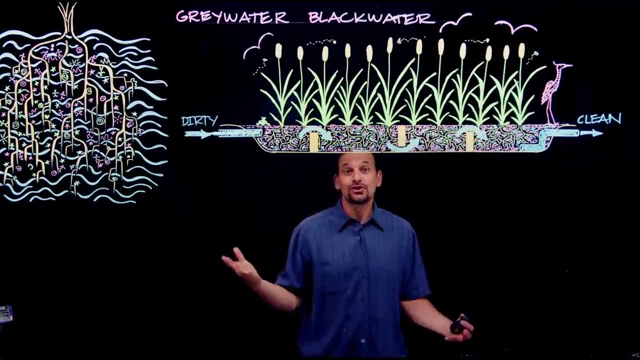 the plant roots And then, at the end of the system, much cleaner water emerges after its time flowing through this big plant filter. So it's super basic, Just a liner, gravel, pipes and plants, And it's all about maximizing the contact between the water and the 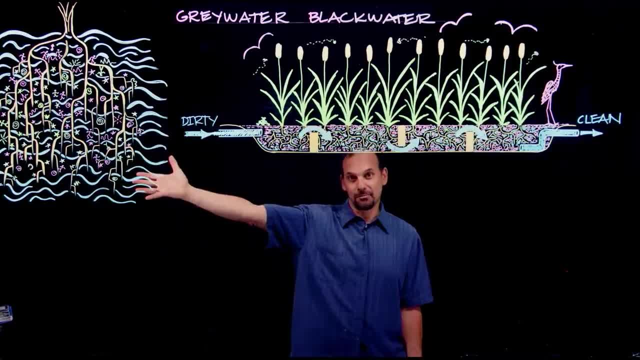 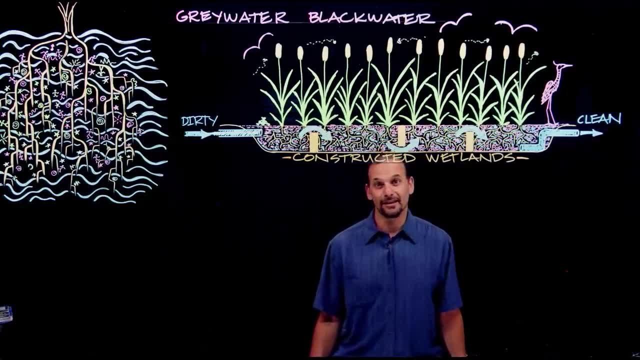 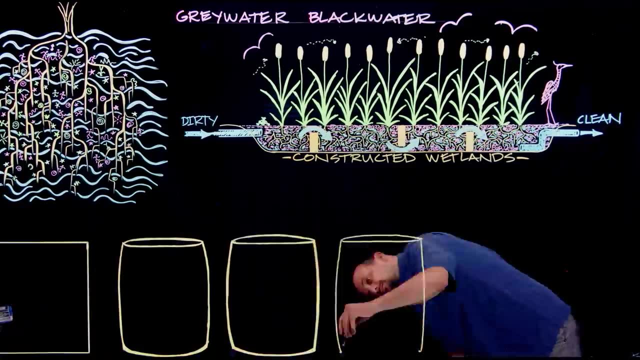 plant roots to get the effect of this awesome party that goes on with the microorganisms on the plant roots. now another really cool system is known as a living machine or an eco machine, which is used to treat black water. in this version of wetland water treatment, the water flows through 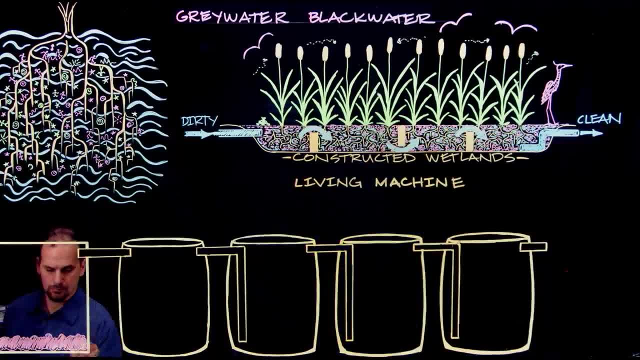 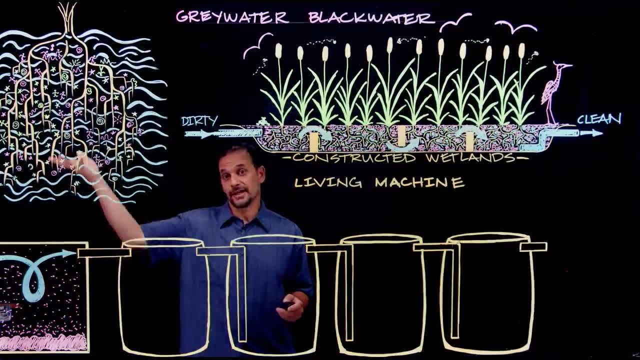 a series of tanks. so for black water it would start in a septic tank to settle out the solids. now this is an opportunity to collect biogas to fuel your kitchen as well. but then from here the water would go into another anaerobic tank, meaning a tank with no oxygen, which helps to further. 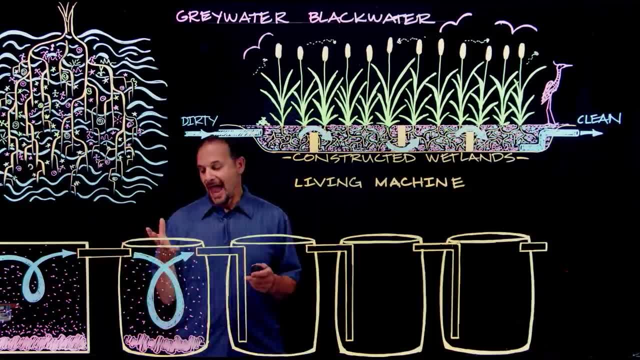 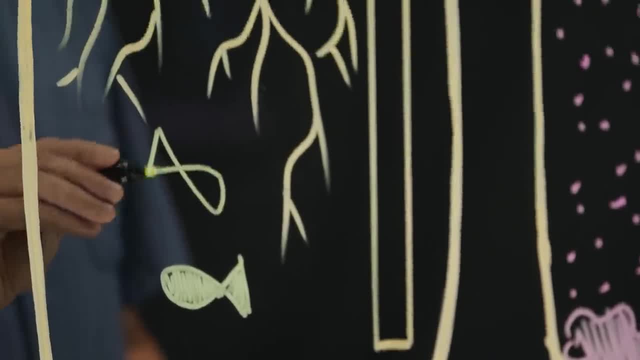 digest the sludge material so from the anaerobic environment. we would then radically change the environment of the water and flow it into a tank full of plants where oxygen is actually pumped in. so there's lots of biological activity in the water and the water would get to filter through all of those. 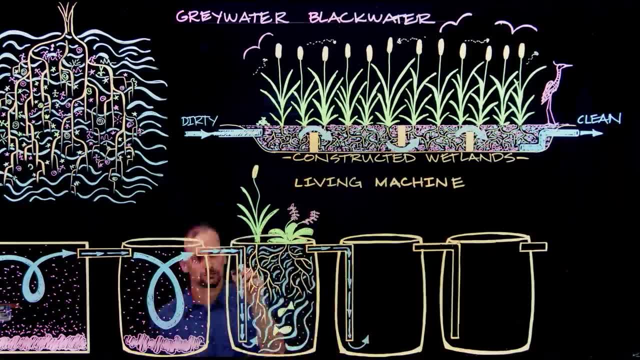 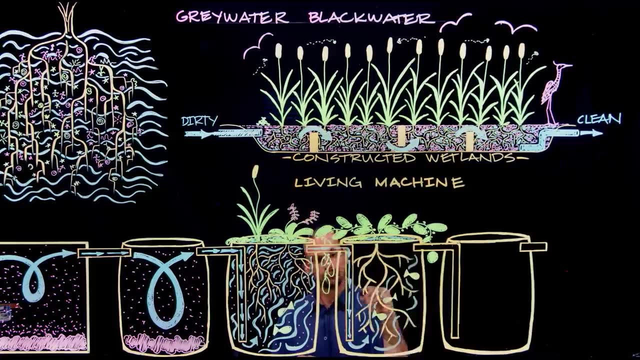 awesome plant roots, like we were talking about here with the party. So the water flows into the bottom and then out the top of each successive tank, where oxygen is pumped in and where all sorts of aquatic plants and animals live. So essentially, the water is being forced through. 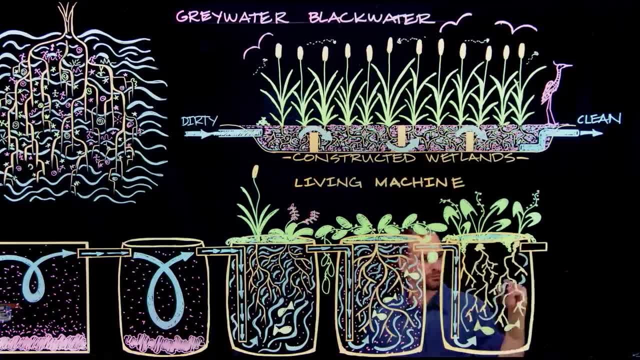 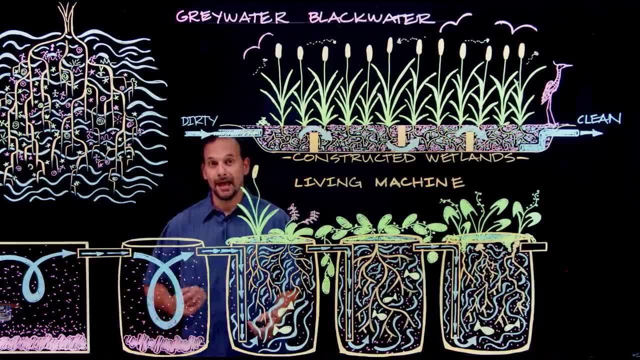 a super biologically active filter and is cleaned along the way. Now, the size of the system depends on how much water is being treated and how many days of treatment it needs to clean the water. So if each of these tanks equals the quantity of water that goes into the system each day, then the 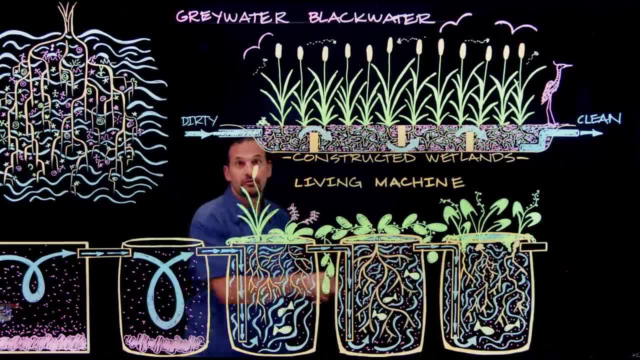 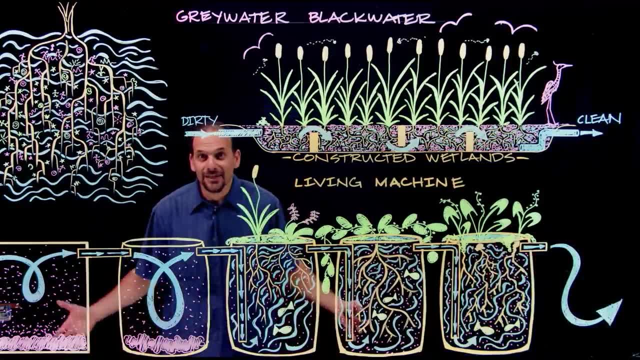 day would receive one, two, three, four, five days of treatment, as the water moves through the entire system from beginning to end. So it's really this simple Biological activity breaks down wastes and absorbs excess nutrients. There are many, many different configurations of these types of systems, so please see the resources. 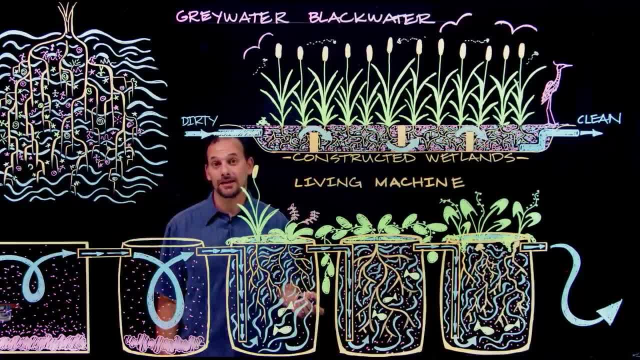 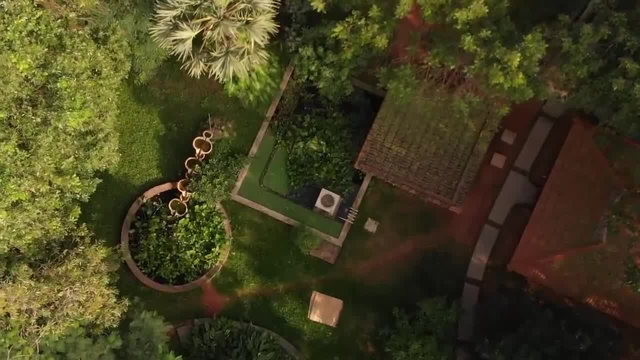 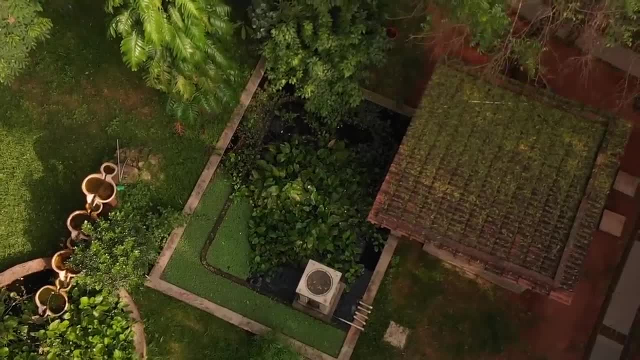 provided in the video description down below for lots, lots more. Here's some footage of a gorgeous living wastewater treatment wetland. I've visited in India and this system handles all of the water from a hotel complex, including toilets, So the dirtiest household waste can be treated with plants and oxygen. But it's even simpler when 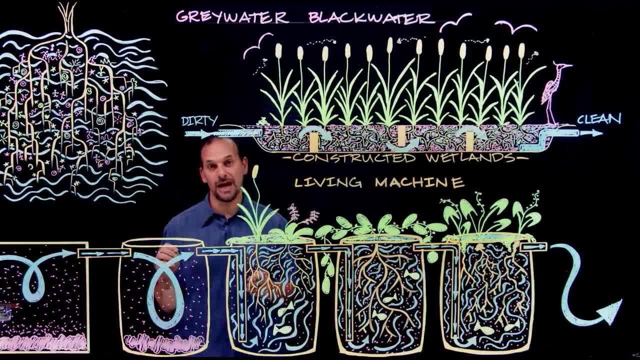 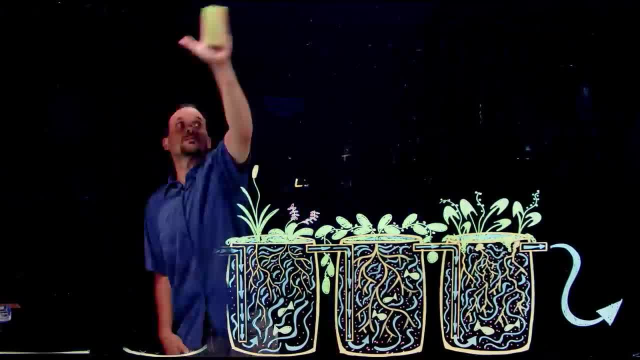 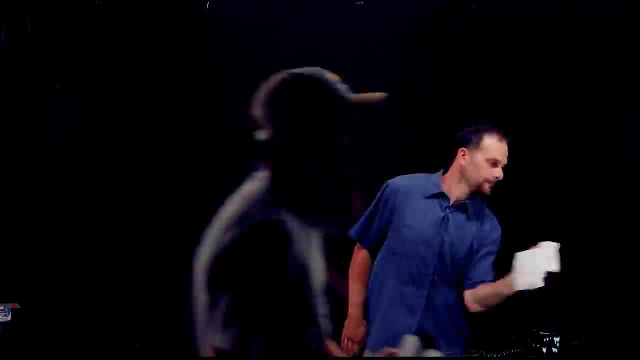 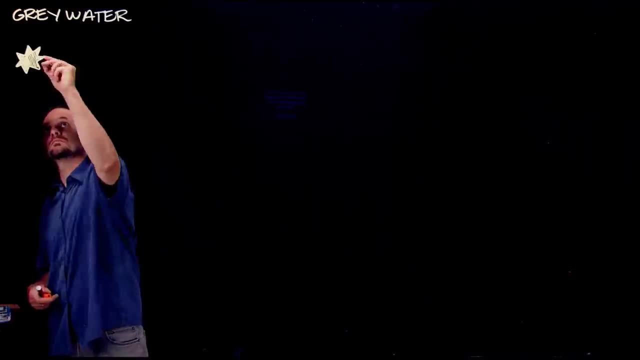 we're treating the barely dirty water coming from showers and laundry. So let's check out some grey water systems. Music, Music, Music, Music, Music Music. The first thing we need to treat most grey water is for the block to contact biologically active soil. 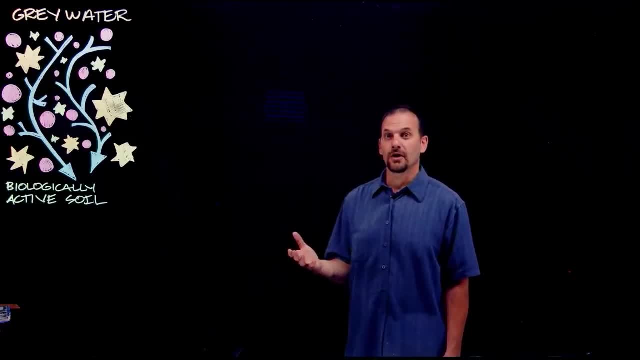 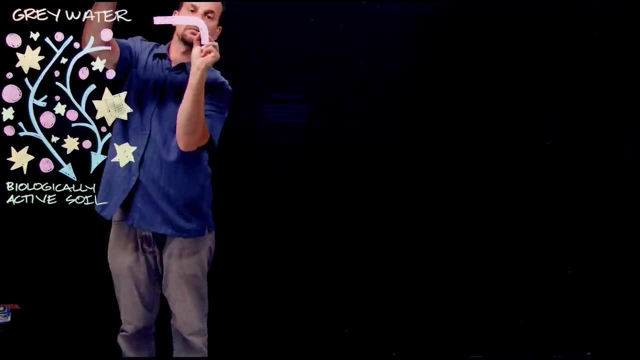 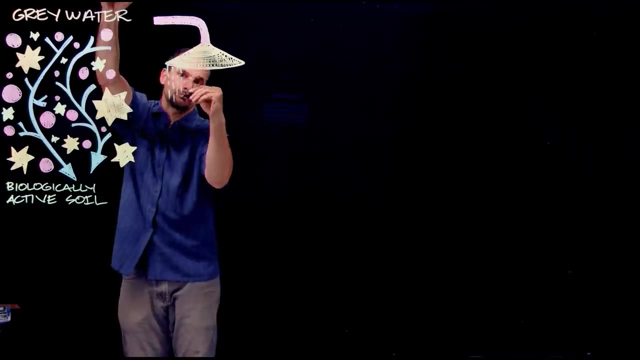 Now. the cleanest and most diluted grey water in our homes, with the highest volume, comes from shower, bath and laundry. The kitchen and bathroom sinks often have pretty concentrated pollutants and may require a grease trap, so they're not really the easiest sources of grey water to recycle. 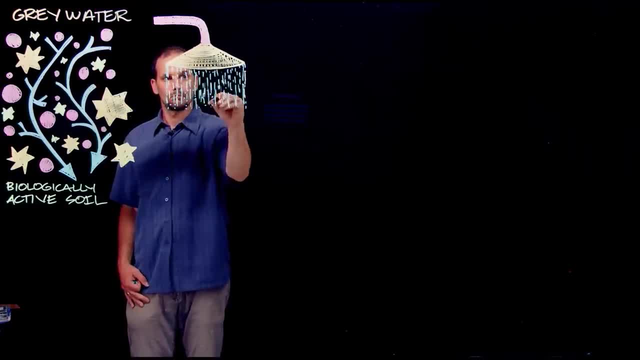 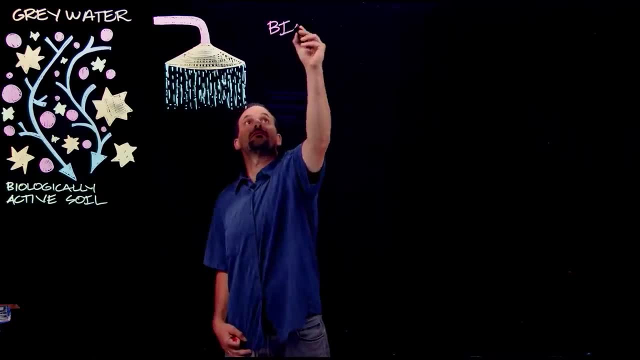 and may be better categorized as black water. Now you need to consider what is epoxy or non-looking resin. consider what products you're using that are going down your drain and into your greywater system. There are biodegradable cleaning products and bath products, and 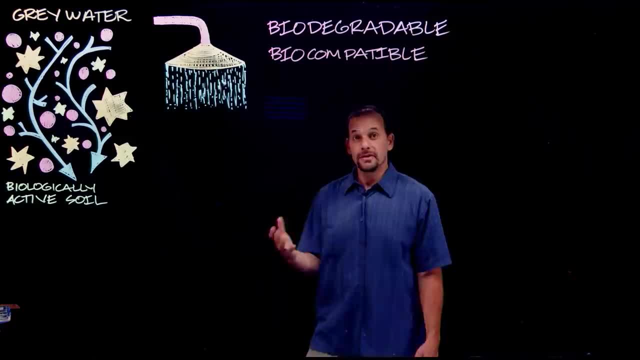 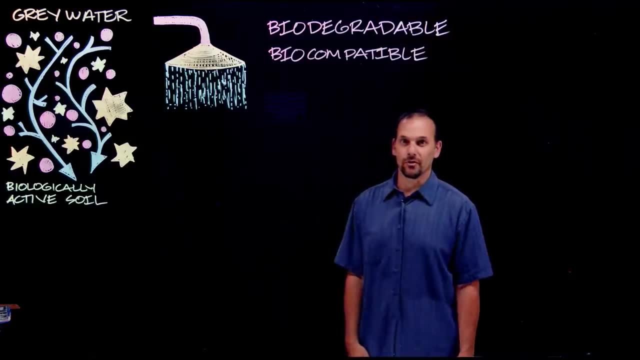 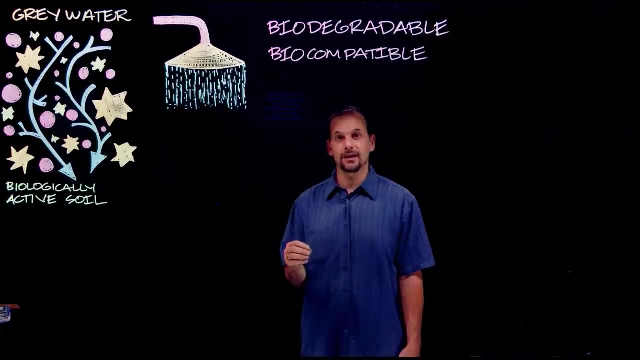 there are also biocompatible products. This means that there are products that will break down, biodegradable, but aren't necessarily good for plant growth, like those containing a lot of sodium, which is salt. Now, biocompatible products actually break down into elements that are beneficial for plant growth. Check the 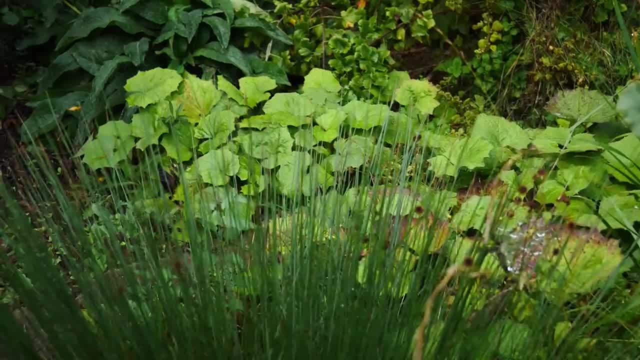 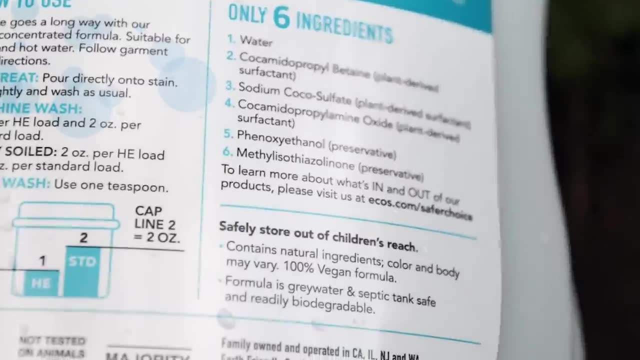 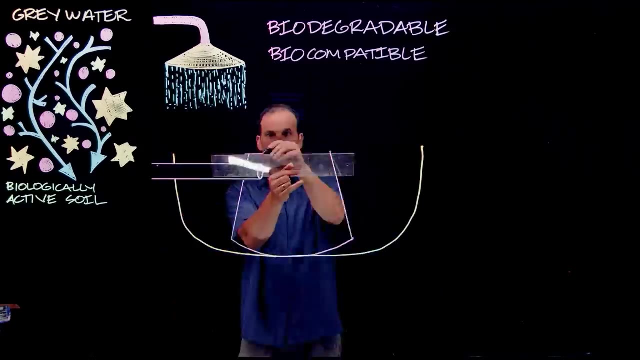 video description for a link to a suggested brand. Here's my laundry system thriving with luscious plants, and you can see on the back of my laundry detergent it specifies that it's greywater safe. There are so many different variations on greywater systems, but my very favorite is the. 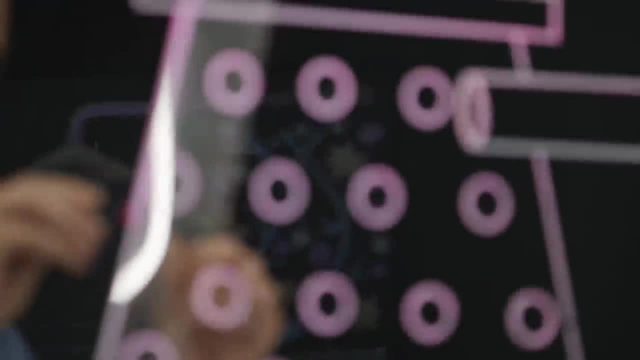 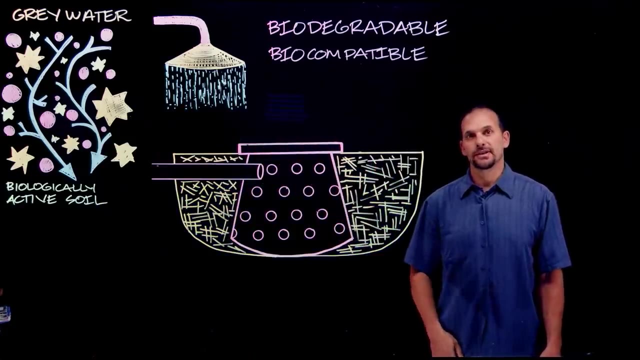 branch drain greywater system that was created by a guy named Art Ludwig and check the description below for a link. Now the greywater is split from its source into various outflow outlet points, and each outlet pipe flows into a bucket with the bottom cut out and holes drilled.